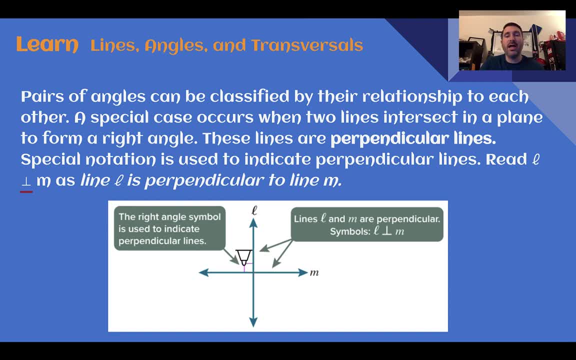 lines usually have a little box in the corner that helps indicate that it is perpendicular or that it forms a right angle. So if we see that, we're gonna know that that angle is perpendicular or 90 degrees. Two lines that never intersect are called parallel. 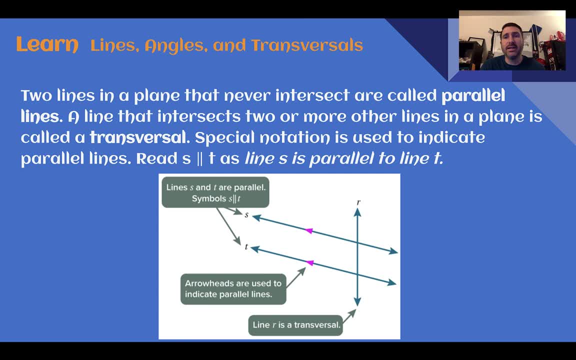 lines. A line that intersects two or more other lines in a plane is called a transversal, And then special notation is used to indicate parallel lines. We see this symbol right here, Similar to perpendicular, where we can see they're crossing. you're gonna see two lines that do not cross And this is read as line S. 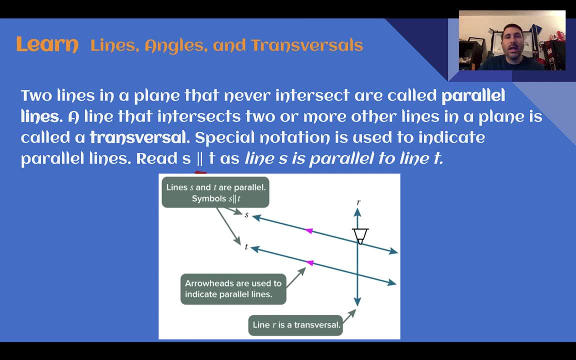 is parallel to line T. If we're given a picture, many times we will see these little arrowheads showing which things are parallel And that's going to be helpful to look for, as parallel lines have specific angle properties. And then a line that's cutting across two or more other lines, that is called a. 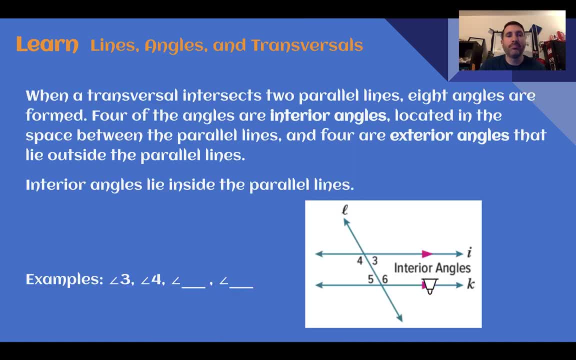 transversal. So line R here is a transversal. When a transversal intersects two parallel lines, eight angles are formed And these angles have special relationships. So four of the angles are interior angles, And when we say interior we mean they're located. 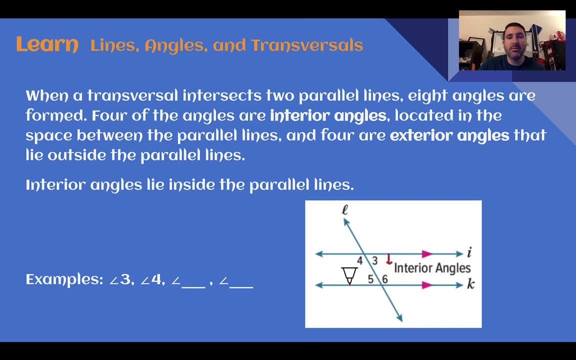 between the parallel lines, So interior, between the two parallel lines. There are also four exterior angles that are outside the parallel lines. So our interior angles, here we have three, four, five and six. They are the four angles that are inside the parallel lines. 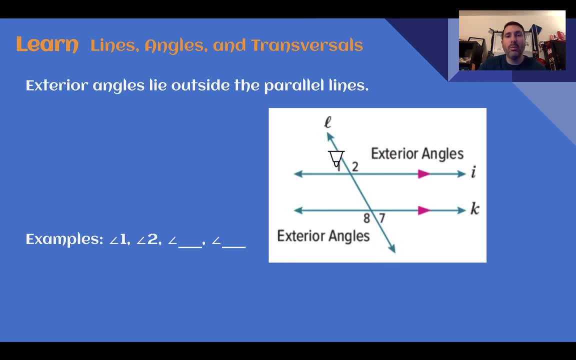 The exterior angles that are outside the parallel lines one and two. And then on the other side, outside the parallel lines, we have angles seven and eight. So we have interior that's inside or, between them, exterior that is outside, And those words are going to be important to know as some of the angles 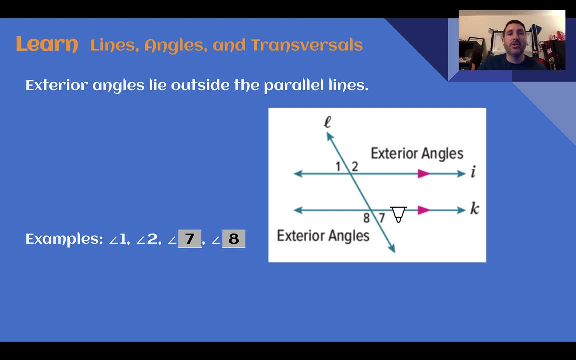 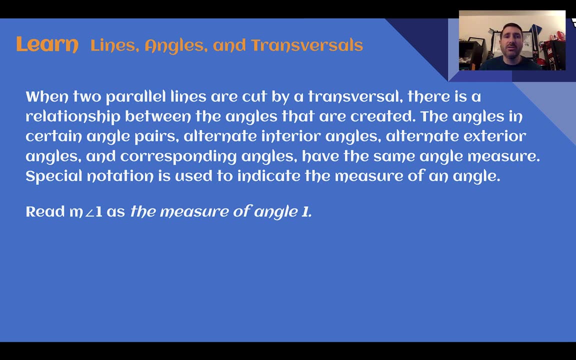 are named those, And it helps you to determine the location of those types of angles. When two parallel lines are cut by that transversal, there's also relationships between the angles that are created Depending on where these angles are located and which pairs we're talking. 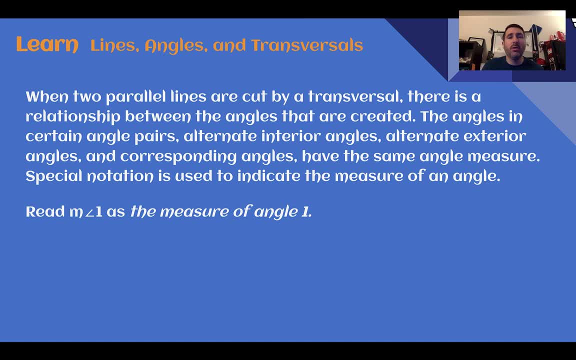 about we could have alternate interior, alternate exterior or corresponding angles. Those angles are going to have the same angle measure And when we're talking about angle measure, we have a special notation written like this: We have M and then an angle That stands for the measure of angle, and then whatever. 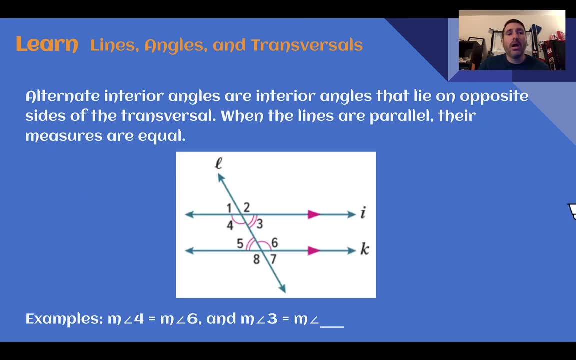 we're talking about So here. this is the measure of angle one. Alternate interior angles are interior angles that lie on the opposite side of our transversal. The name gives us a little bit of a clue about where the angles are located. I'm going to start with the word interior. 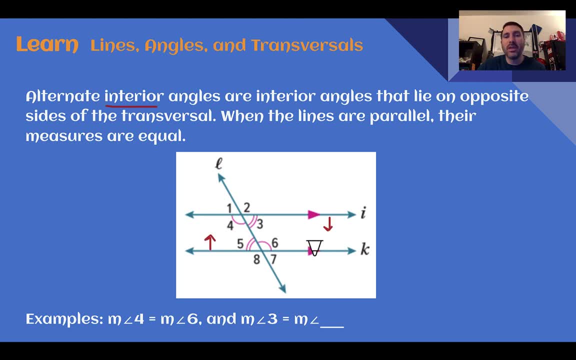 Interior again, meaning inside our parallel. So we're looking at angles three, four, five and six For alternate. we're looking at opposite sides of the transversal, But not only that kind of like the opposite corners. So angles four: 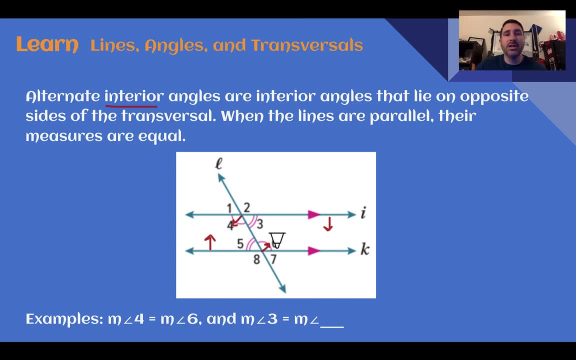 and six are alternate interior angles. The same would be angle three and angle five. These angle pairs have equal measures, So the measure of angle four is the same as the measure of angle six. Angle three and angle five have the same measure, meaning they are the same sized angle. 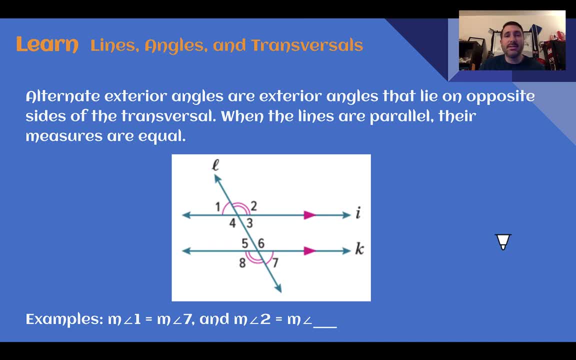 Alternate exterior angles work pretty much the same way as the interior ones, but they're on the outside. We have exterior. So outside of the parallel, The alternate part, they're still opposite to the transversal. So angle one, Angle 1, is alternate exterior with angle 7.. 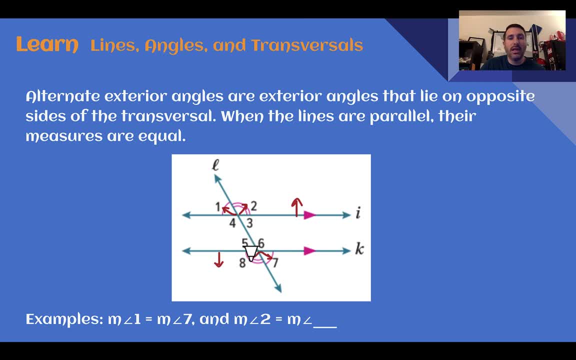 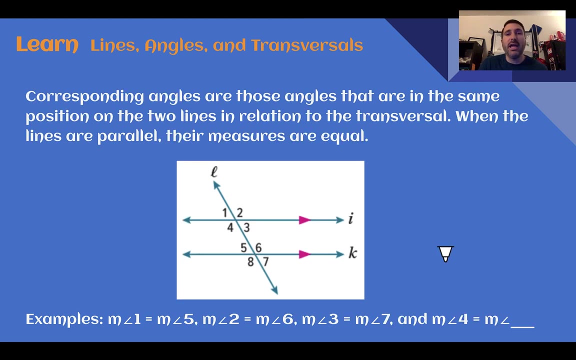 Angle 2 is alternate exterior with angle 8. Again, those angle pairs have the same measure. So angle 1 has the same measure as angle 7.. Angle 2 has the same measure as angle 8.. A third type of angle pair that's formed are called corresponding angles. 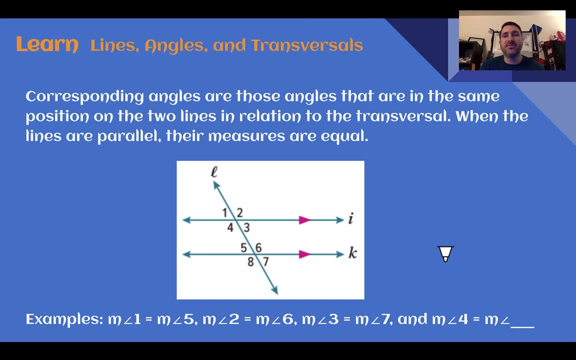 They are in the same position on the two lines in relation to the transversal. When the transversal cuts parallel lines, they also have equal measures. So in this case we have angle 1 and angle 5. They are in the same position relative to the transversal. 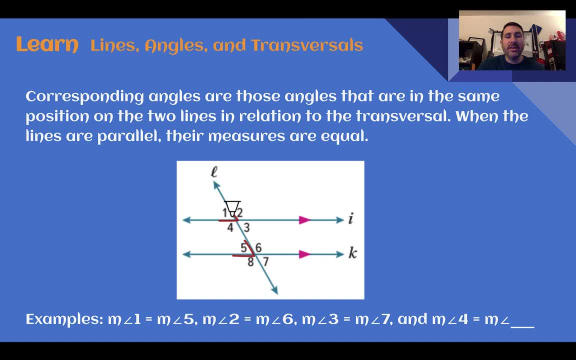 One's just on one parallel line, the other's on the other. Following that same thing, angle 2, angle 6 have the same measure. Angle 3 and angle 7 are in the same position, so they have the same measure. 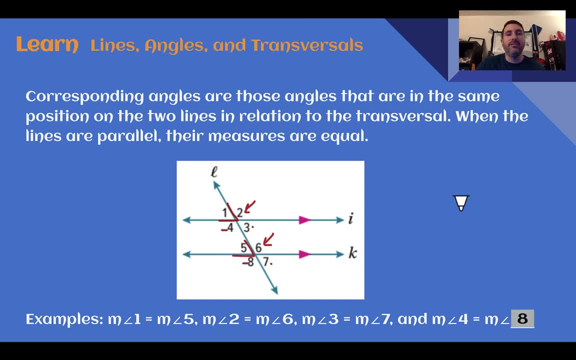 And angle 4 with angle 8.. They have the same measure. So if they're in the same position they are called corresponding angles and they also have the same measure. So all the ones we just looked at- alternate interior, alternate exterior and corresponding. 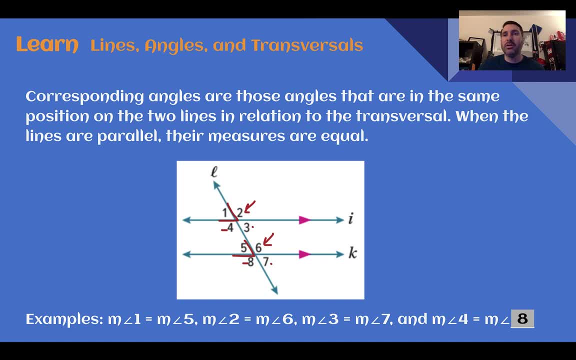 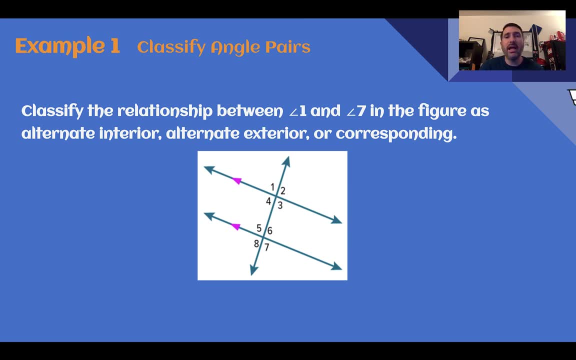 they are all equal when we're talking about the pair of angles. Example 1, classify angle pairs. Classify the relationship between angle 1 and angle 7 in the figure as alternate interior, alternate exterior or corresponding, or we really should take into the fact that it could. 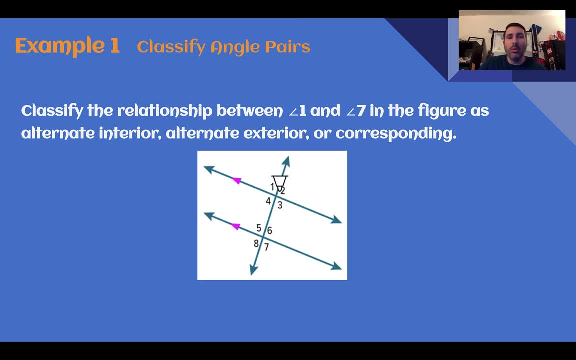 be none of these. So first let's locate angle 1,, which is right here, and angle 7,, which is right here. The first thing I notice they are outside the parallel lines, So right away I know that they are exterior. 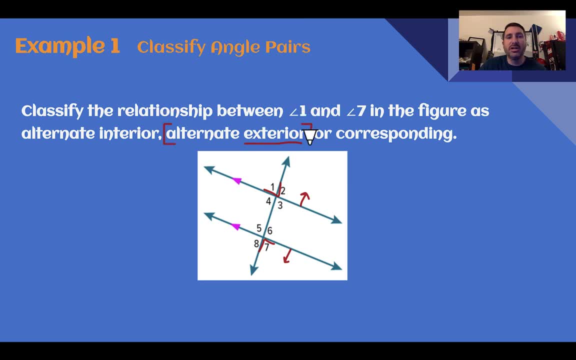 So exterior, it's probably either alternate exterior or the reason I said it could be none is because you can have things that are exterior, that are not alternate exterior, And they wouldn't be corresponding either, because they wouldn't be in the same position. 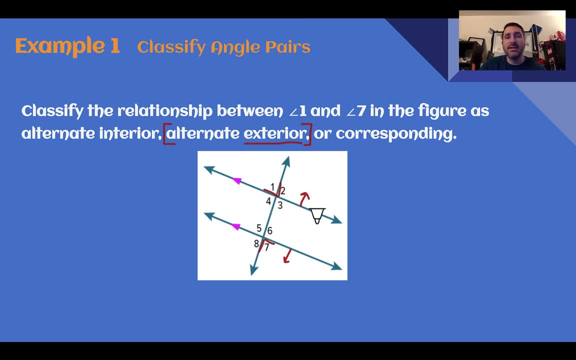 So these are exterior. Are they alternate exterior? They are on opposite sides of our transversal there. So, yes, these are exterior angles that are on opposite sides of the transversal, So they are alternate exterior angles. If we were given 2 and 7, even though they are exterior, they're not opposite sides of. 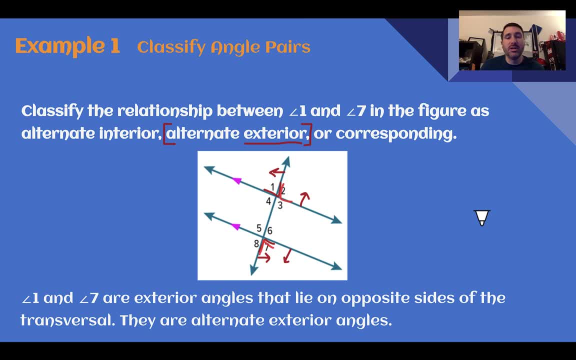 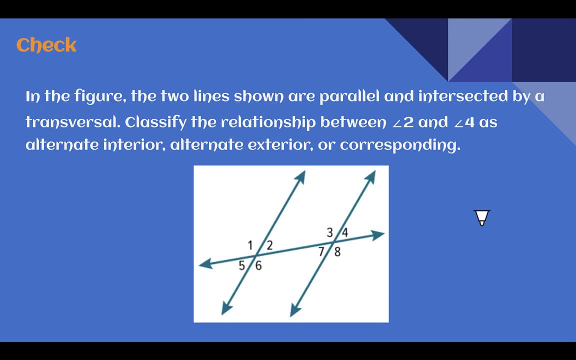 the transversal. So that would be an instance where it would be none of the types. So be careful that it fits both criteria for the type that you're looking at. Check your understanding, read through the situation and classify the angles given as. 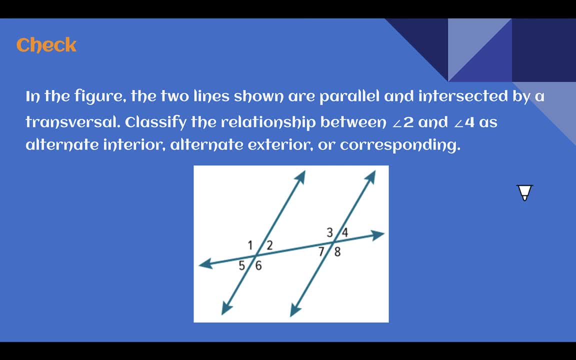 alternate interior, alternate exterior or corresponding. Pause the video now and complete the check. Check your answer. You should have said these are corresponding angles. Okay, Here's angle 2,, here's angle 4.. So our first step is to locate them. 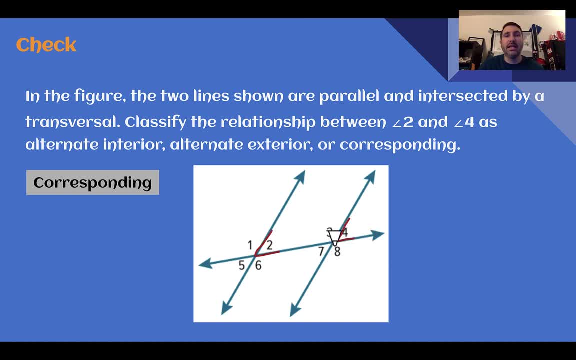 They are in the same position relative to the parallel lines and the transversal, So that makes them corresponding. They're not both inside, so they can't be alternate interior. They're not both outside, they can't be alternate exterior. These are corresponding. 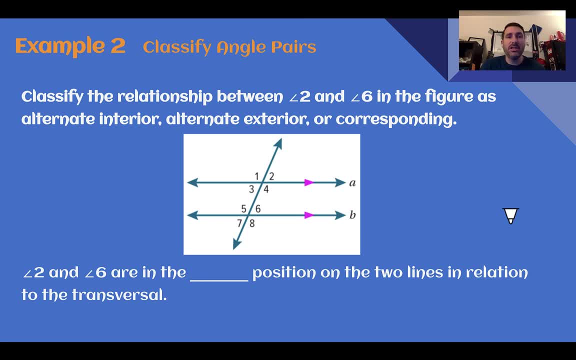 Example 2. Classify angle pairs. Classify the relationship between angle 2 and angle 6 in the figure as alternate interior, alternate exterior or corresponding, Or again could be none of them. Let's find angle 2 and 6.. 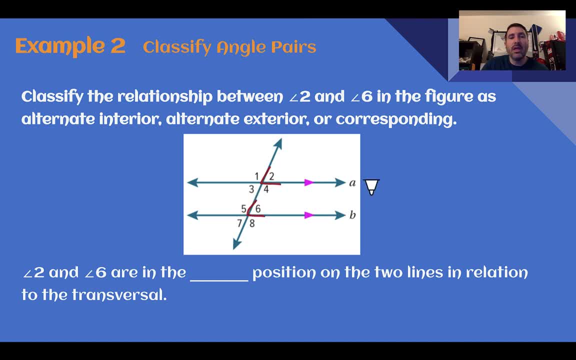 So here's angles 2, here's angle 6.. Angle 2 and angle 6 are in the same position in relation to the transversal. So, just as we saw in our check, these are corresponding angles. It's like we took one of the angles and we were able to just move it and it fits perfectly. 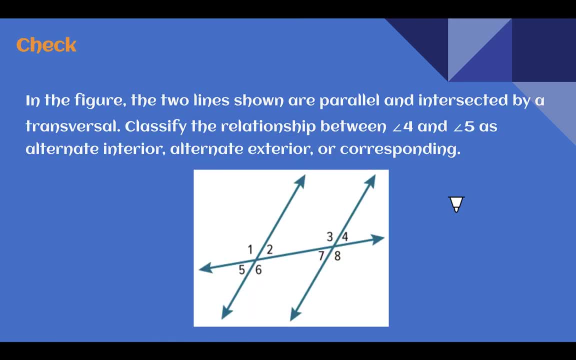 on top of the other, No rotations or anything. Check your understanding. What would angle 4 and angle 5 be considered? Pause the video now and complete the check. Check your answer. These are alternate exterior angles. So here's angle 4, here's angle 5.. 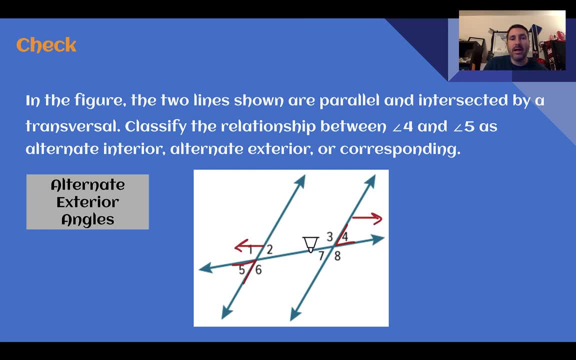 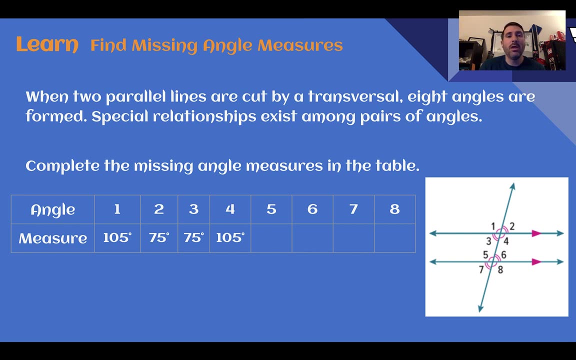 They are outside the parallel and on opposite sides of the transversal, so these would be alternate exteriors, Exterior angles Outside for exterior, opposite for alternate. Let's learn Find missing angle measures. When two parallel lines are cut by a transversal, eight angles are formed. 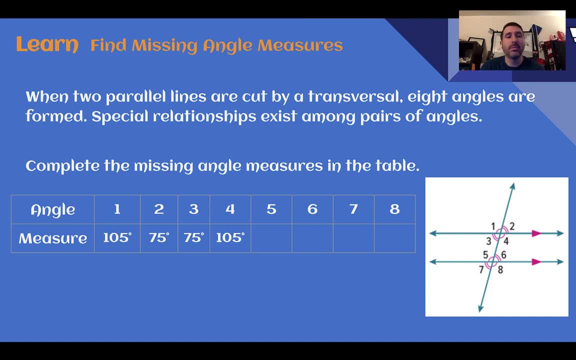 Special relationships exist amongst the pairs of angles. Complete the missing angle measures in the table. So first we're saying angle 1 is 105,, angle 2 is 75, angle 3 is 75, angle 4 is 105.. 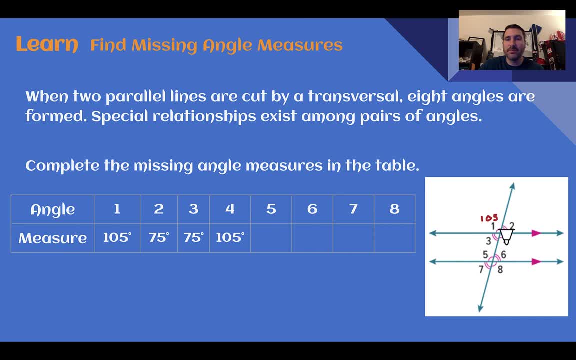 So I'm going to fill that in over here, just so we can see how this works. Angle 1 and 4 were 105,. angles 2 and 3 were 75. We can use any of the three angle relationships we were just talking about. so alternate interior. 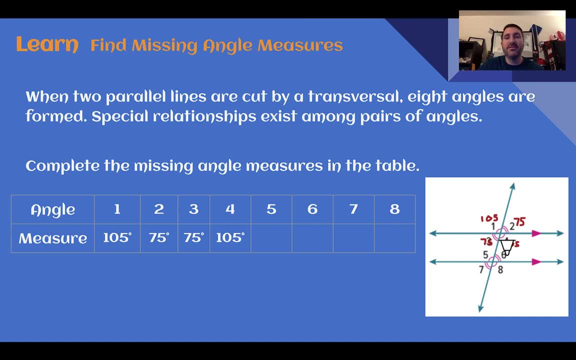 alternate exterior or corresponding to figure out what 5,, 6,, 7, and 8 are equal to. If I want to use corresponding angles, I can say: angle 1 has the same measure as angle 5, so that would also be 105. 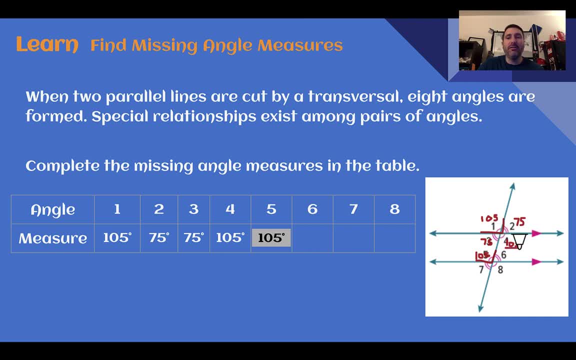 I also could have used alternate interior. Angle 4 would be the same as angle 5, and again I still would have found that it was equal to 105 degrees. I can do the same thing with angles 2 and angle 6, using corresponding to find that. 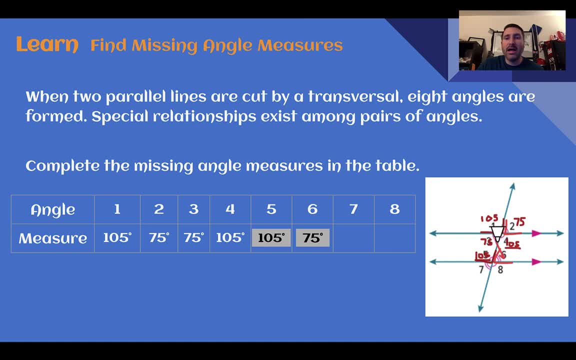 angle 6 is 75.. Or I could have done alternate interior angles, Again with angle 3, and still found 75.. For angles 7 and 8, we can use alternate exterior angles. So 1 would be an exterior with 8, meaning this is 105. 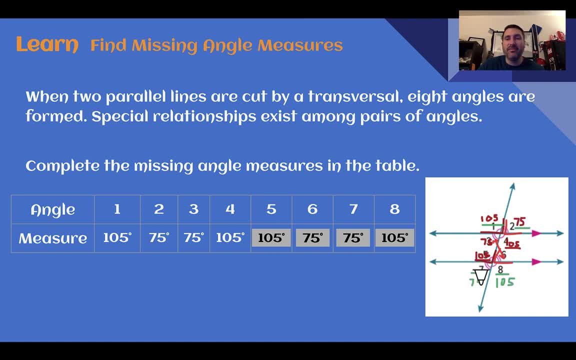 2 would be an exterior, with 7, so that would be 75. Or I could have used corresponding Angle 4 goes with angle 8. Angle 3 goes with angle 7.. There are a bunch of different ways. using any of the three methods we can figure out. 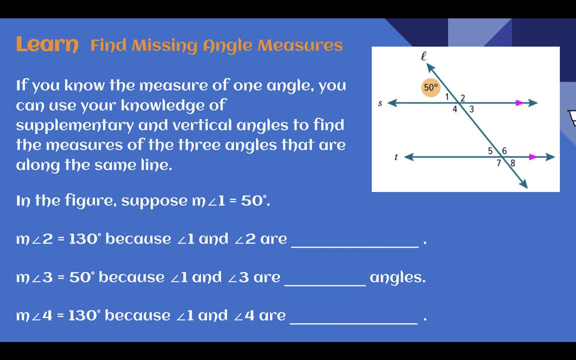 the missing measures of angles. In addition to the three angle pairs we just looked at, if we know the measure of one angle, we can also use our knowledge of supplementary and vertical angles to find the measure of the three angles. along the same line, 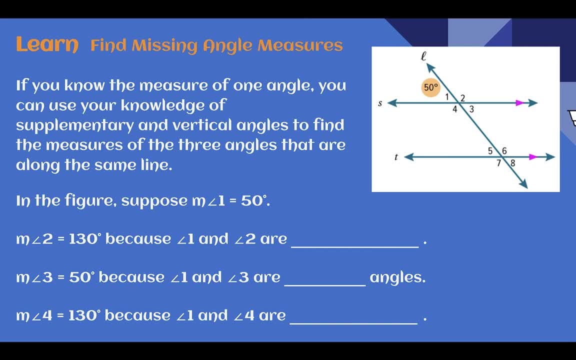 We're not really going to see complementary angles unless we're dealing with a perpendicular line, which most of the time it's not So if we're given in our picture, angle 1 is equal to 50 degrees, We can quickly figure out angle 2 is equal to 130 degrees, because angle 1 and 2 are 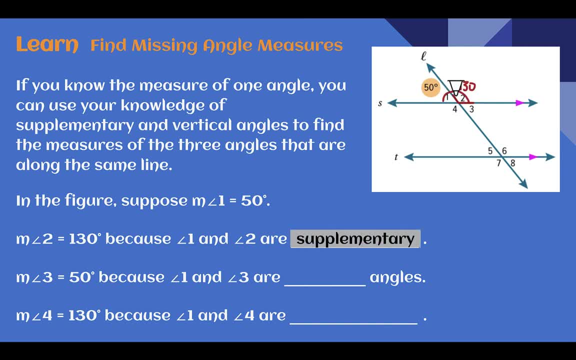 supplementary. They make a straight angle. when put together, they are supplementary and supplementary adds to 180. We can figure out angle 3, because angle 1 and angle 3 are vertical angles. Vertical angles were the ones that are directly across from each other when two lines intersect. 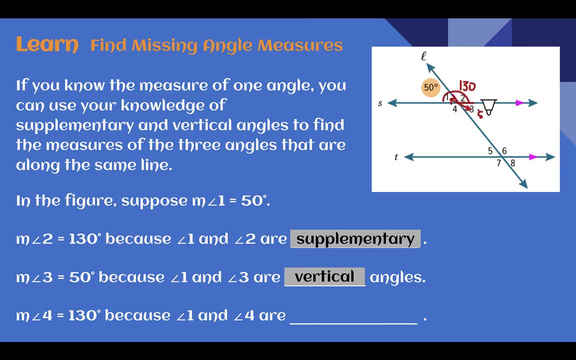 They have the same measure. So if 1 was 50, then 3 is 50.. For angle 4, we can say: angle 1 and angle 4 are also supplementary, so that would be 130 as well. Or now that we knew, angle 2,, angle 2 and 4 were vertical, so that would be equal. 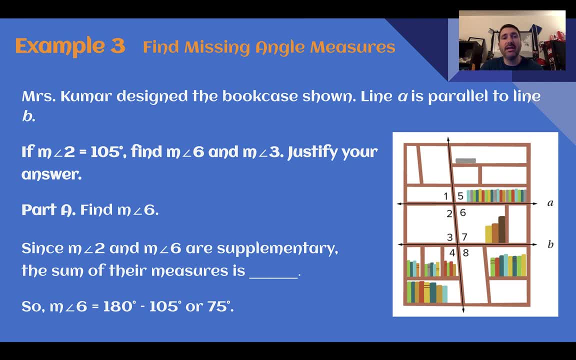 Example 3, find missing angle measures. Mrs Kumar designed the bookcase shown. Line A is parallel to line B. If the measure of angle 2 is 105 degrees, find the measure of angle 6.. And the measure of angle 3,? justify your answer. 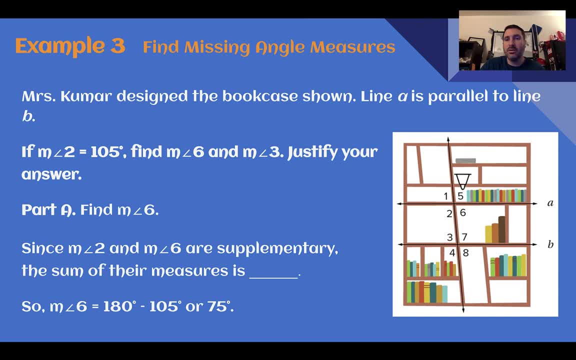 So part A, let's find the measure of angle 6.. So here's angle 6. We need to be able to find that angle. What we're given is angle 2 is 105.. Notice, angle 2 and angle 6 together make a straight angle, so they are supplementary. 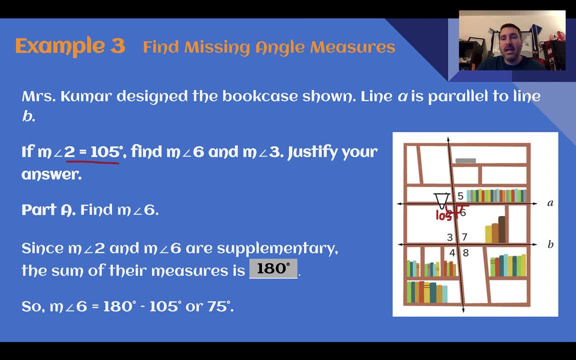 meaning if we add them together, we get 180 degrees. If angle 2 is also a straight angle, we get 180 degrees. So the answer is angle 3.. If angle 3 is 105 degrees, we get 75 degrees. 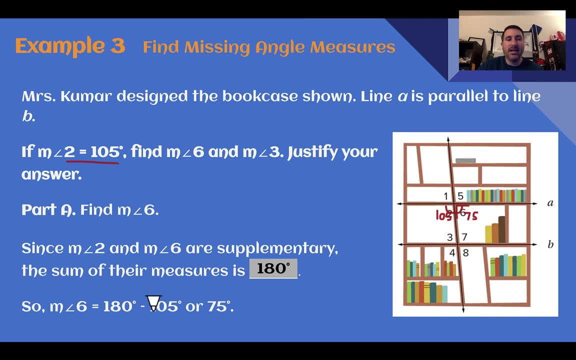 If angle 6 is also a straight angle, we get 80 degrees, So we get 75 degrees. So if the measure is already 105, then angle 6 must be 75. I get that by subtracting. I take away the measure I know from 180 and I'll get what's left. 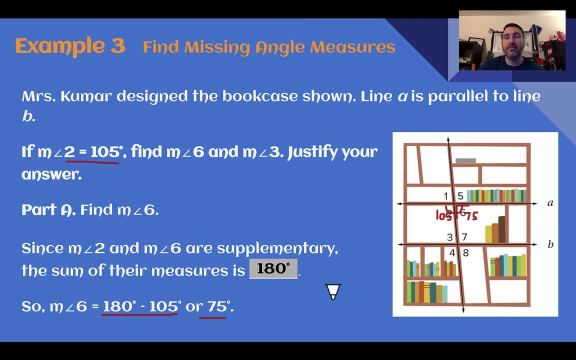 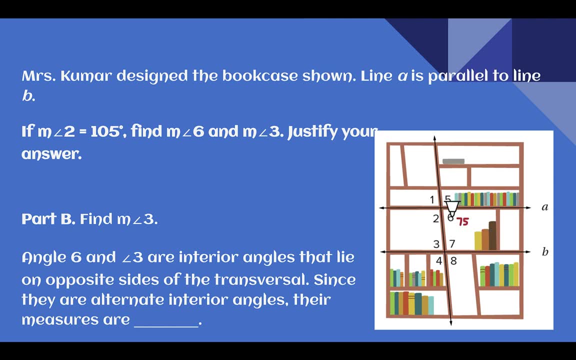 So 180 minus 105 tells us our missing angle was 75. So that's our measure for angle 6.. Next let's find the measure of angle 3.. So I rewrote that measure of angle 6 was 75.. 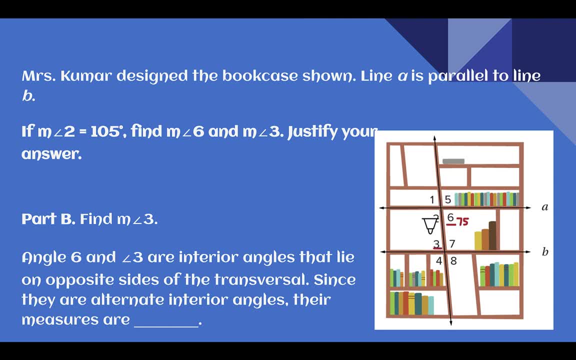 We can see now that six and three- the other one I want to know- have a higher value than have a special relationship that we just looked at. They are alternate interior, So inside the parallel, and they are opposite corners, opposite of that transversal, Since they are alternate. 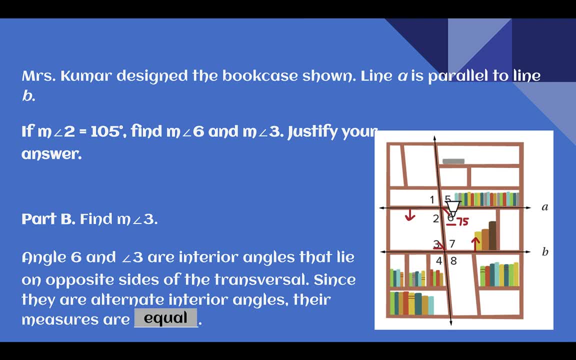 interior angles. their measures are equal. And if they're equal, since measure of angle 6 is 75,, then the measure of angle 3 also must be 75. So 75,. both angle 6 and angle 3 were 75 degrees. 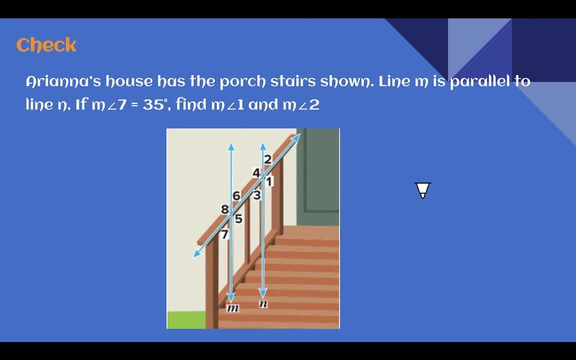 Check your understanding. Find the measures of angles 1 and 2.. Pause the video now and complete the check. Check your answer. You should have found angle 1 is 145 degrees, while angle 2 is 35. So let's pull it out. 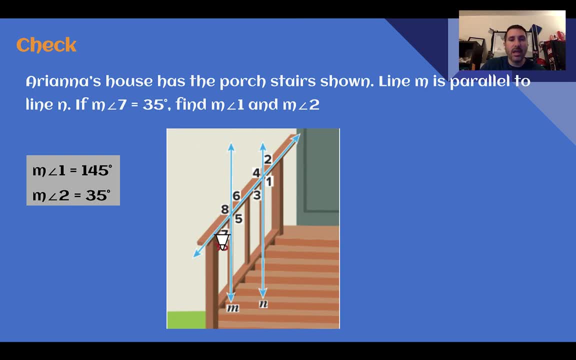 Plug in what we know. Angle 7 down here is 35.. I'm looking to figure out angle 2 and angle 1.. Here, angle 7 and angle 2, they are alternate exterior angles Outside the parallel opposite sides of the transversal. So this one's on this side, this one's on this side. 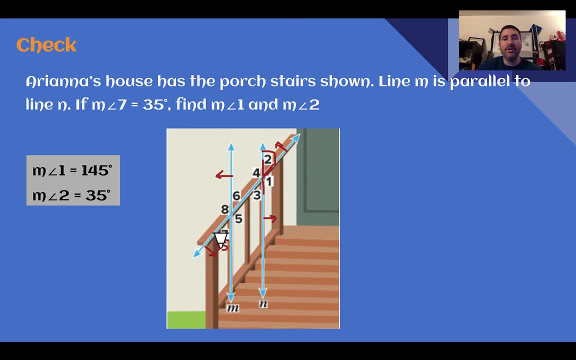 Alternate exterior angles are equal. So if 7 is equal to 35,, then 2 is also equal to 35. Which is what they said. Then angles 2 and 1, they form a straight angle, meaning they are supplementary. So 180, take away 35, and I end up with 145. 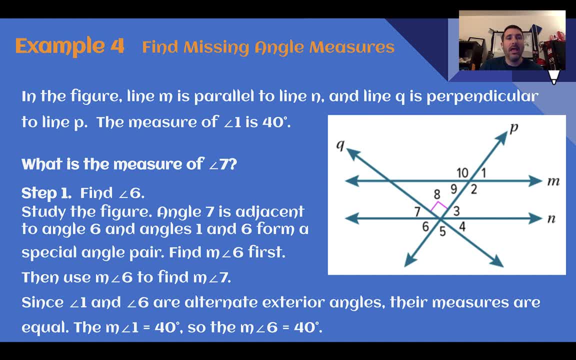 Example 4.. Find missing angle measures In the figure. line M is parallel to line N and line Q is perpendicular to line P. The measure of angle 1, is 40 degrees. What is the measure of angle 7?? This picture looks pretty complicated. 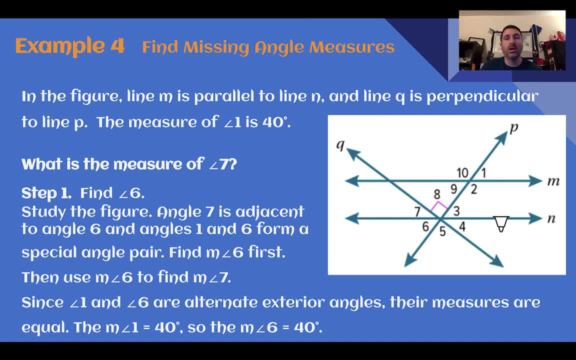 but if we fill in our angles as we go, we can start to work our way towards angle 7.. So we know angle 1 is 40. So I'm going to put 40 in that place. We also know the measure of angle. 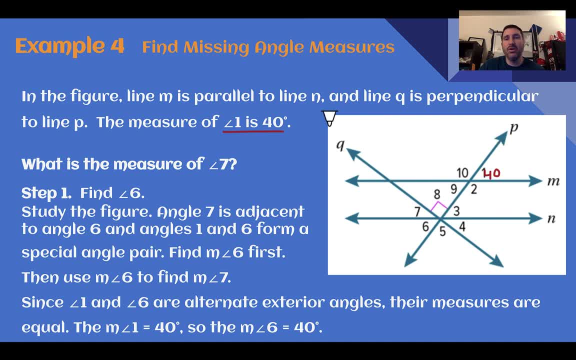 8. They gave us this little box here and told us that Q is perpendicular to P, So this is 90. Angle 7 is what we are trying to get to, So let's start filling in stuff around it. To get to angle 7, let's look at our diagram and see if we can figure out the quickest way. 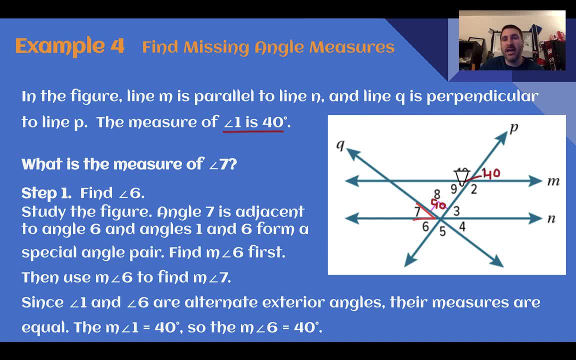 to get there. I could go across and say that 40, angle 9 must also be 40. I could make 2 supplementary, But I end up filling in angles that I don't really need. to get there. I can, but they're not necessary. If I look closely, I have angle 1 there. 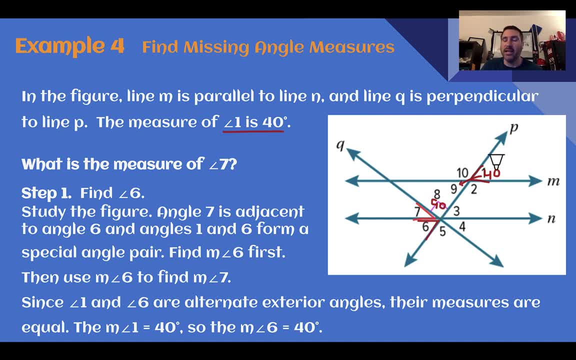 it forms the special relationship with angle 6.. They're outside our parallel and our transversal. that crosses the parallel. this direction is P. So if we ignore line Q, angle 1 and angle 6, they are alternate exterior angles. So if angle 1 is 40, then angle 6 is also. 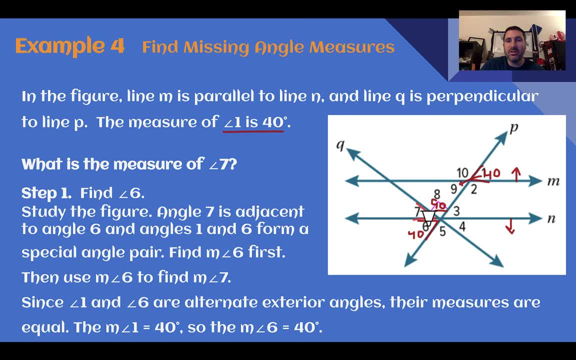 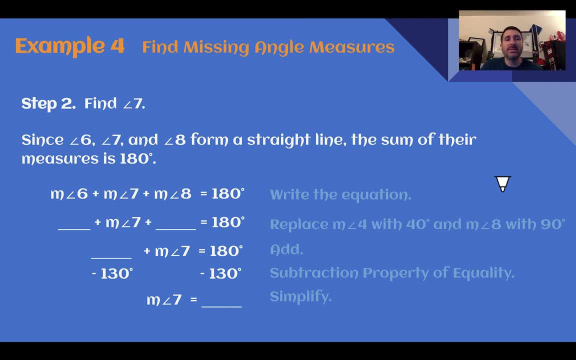 40.. Once we know that these three angles together make a straight angle, so they would add to 180.. Since 6,, 7, and 8 add to 180, we would add their measures together to equal 180.. 6 was 40,, we just figured that out. Angle 8 was our right angle, so that was 90. 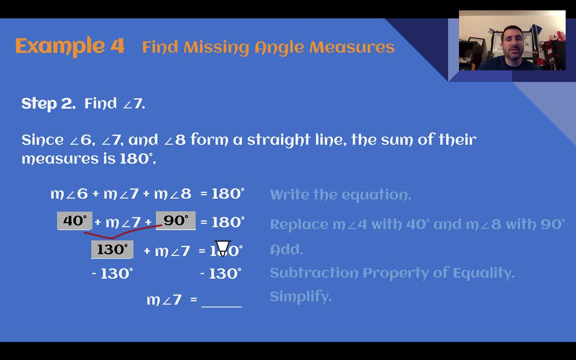 Combine these two together, that's 130 degrees. So we have to find the measure of angle 7.. What's left to get to 180.. Take away what we already have. measure of angle 7 is 50 degrees. So this would be. 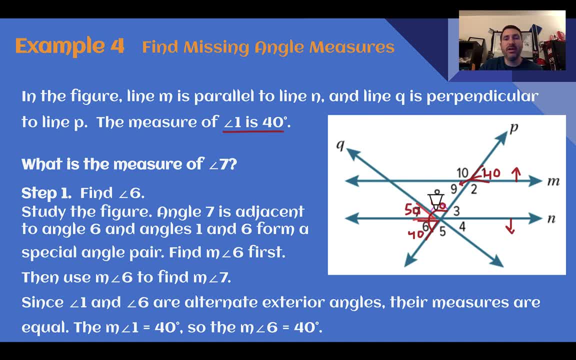 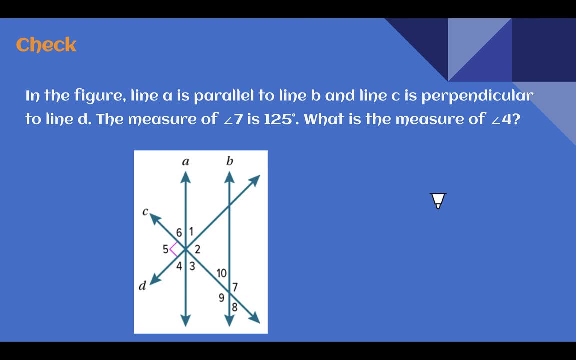 50 degrees here. These three angles here are supplementary and add to 180.. Check your understanding. What is the measure of angle 4?? Pause the video now and complete the check. Check your answer. You should have found that angle 4 is 35 degrees. Let's see if we can figure. 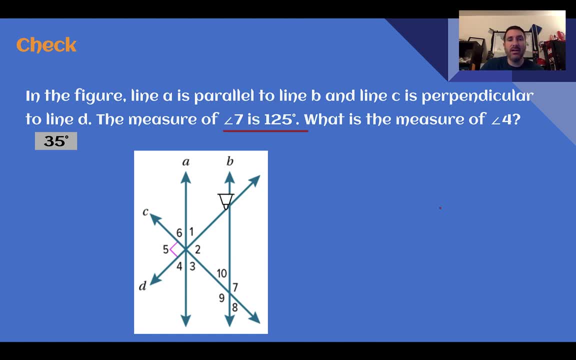 out the most efficient way to get there. It tells us angle 7 is 125.. That's down here And c is perpendicular to d, so we have a 90 degree angle. We also have a 90 degree angle right here, showing that's in the other place where c is perpendicular to d. We want to figure. 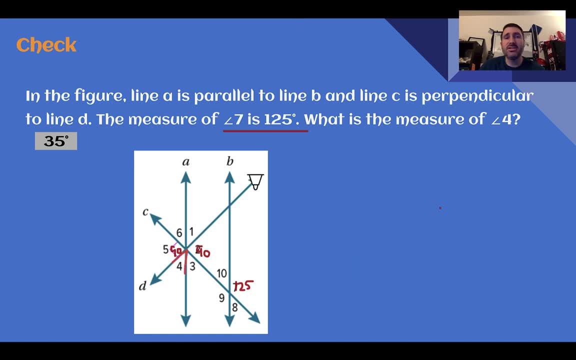 out angle 4.. For this there's a couple different ways that you could do it that are about the same time that it takes. So if I make this supplementary, these two together, then 8 must be 55 degrees, Since those two would add to 180.. Then I could see that angle 8 is corresponding with. 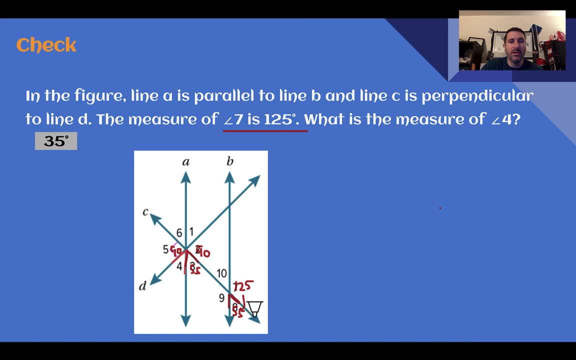 angle 3, so this also would be 55. They're in the same position on our parallel Last. these three angles together 90 plus plus angle 4. Make sure you write the angle symbol here so you don't think it's 4. And 55. Those three added together: 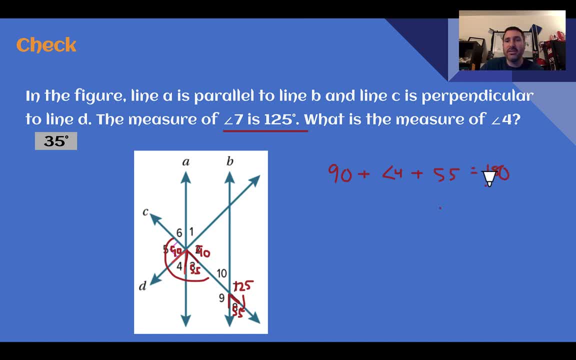 If I take away 90, and take away 55, so I just took away both of those- I'm left with 35 degrees. So the measure of angle 4 is 35 degrees. There are other ways to get there. Maybe you noticed this angle here. they are vertical. Then it would correspond to this: angle here. with both of those together, 90 plus 1. That would be 55 degrees If I take away 90, and take away 55, so I just took away both of those, I'm left with 35 degrees.